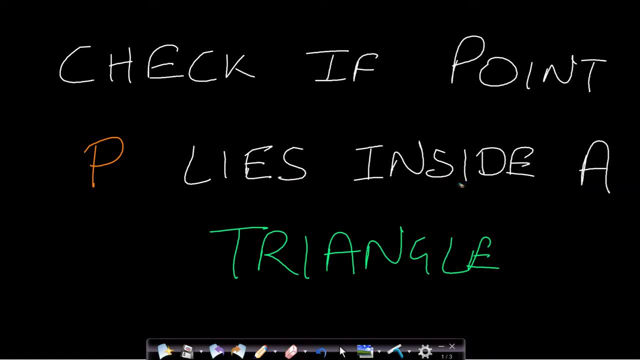 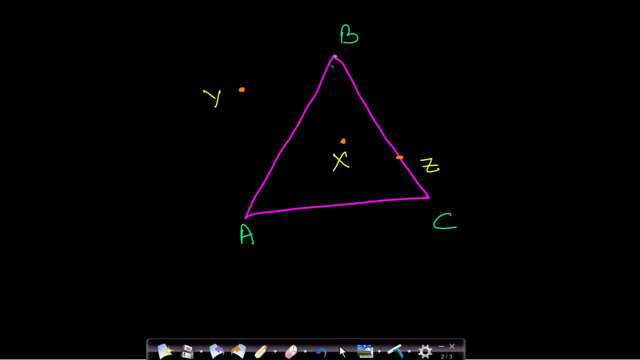 Hello guys, welcome back to TechDoze and in this video we will see a very interesting and a tricky question which is often asked in the interviews, which is to check if the given point lies inside a triangle or not. let me explain you the problem. given a triangle, abc, you want to determine whether 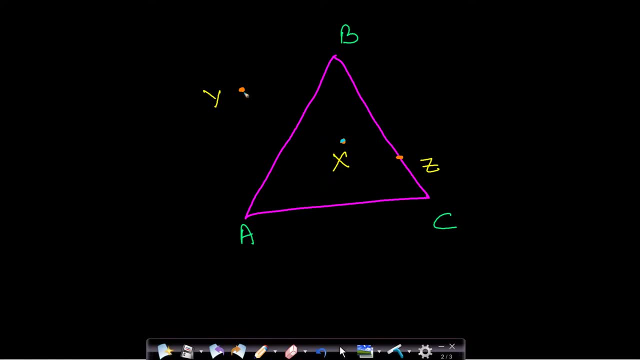 a point x lies inside a triangle or it's outside a triangle. so this is the simple problem statement. i hope you will try it by pausing the video and we will proceed once you have tried this problem. i hope you have tried it by now. so let us look at the solution. let's say we are given the triangle. 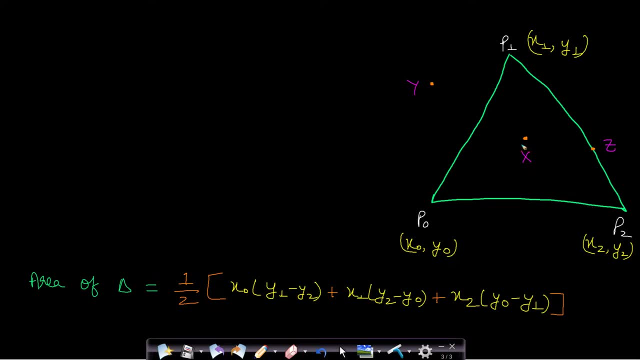 p0, p1, p2, and we are given, like three cases, whether the point lies inside a triangle or outside a triangle or on the triangle line. okay, so how can we determine? a very simple trick is: if you are given a point, let's say we don't know where it lies. we just need to take all these lines as base. 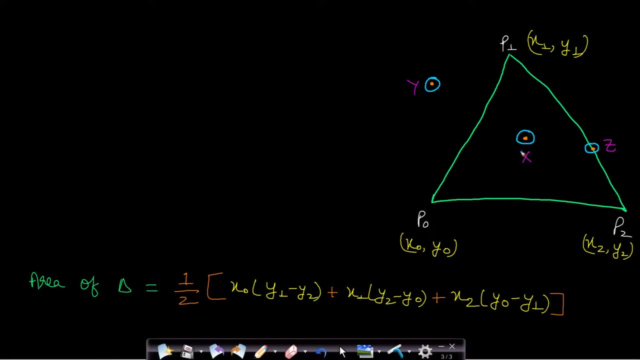 one by one and find the area. so let's say our point is x, then what we will do is we will just make a triangle which is p1, x, p, naught, and then find this area okay, and then we will take this p1, p2 as our base. this is, let's say, base two line. 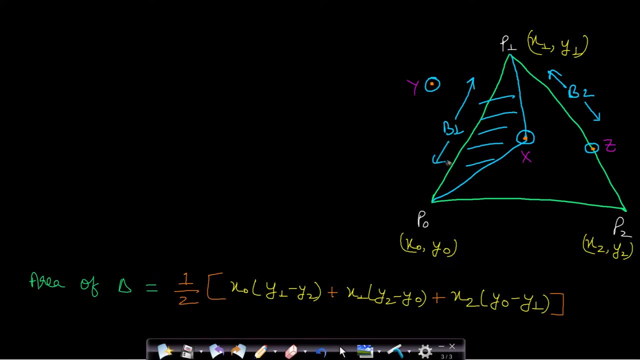 this was our base one line, so we found area, which is area one, using this base one, using this line, base two, we will find this triangle, area, this one- okay, so this area is, let's say, a2. and then, using this base 3, which is this one p naught p2, we will find the area of this triangle. 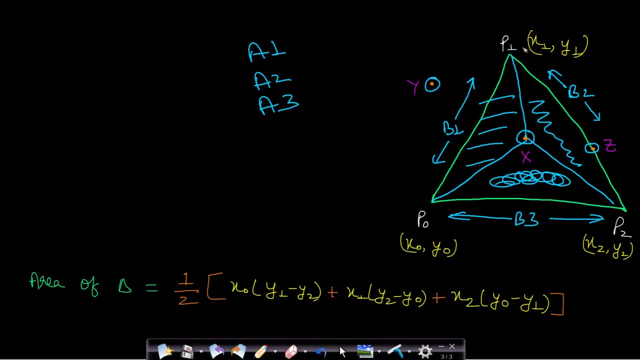 so let's call it a3. now we will also find the area of this entire triangle. now let's call it a if the area of the entire triangle is equals to some of the areas that we found, by using these three vertices as base and this point x as our vertex, then we can safely assume that the point 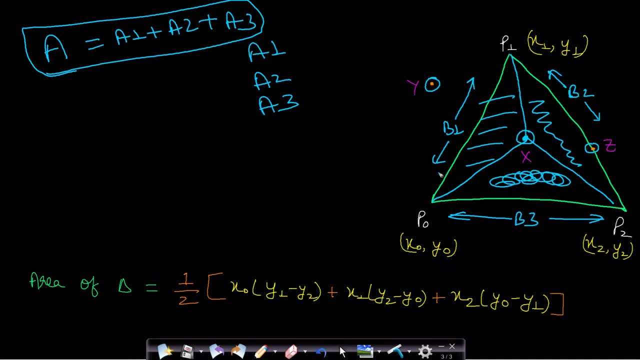 lies either inside or outside the original integral triangle. now let's choose this triangle and Hollow the triangle, or on the triangle. now what happens if our point lies outside the triangle? if you take this base b1 and find this area, this as a1, then you will find that when you take this base 3,